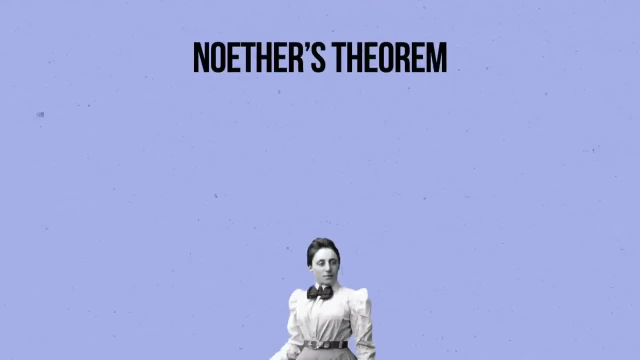 A couple of videos ago we learned about Noether's theorem, one of the most profound results in all of physics. that says that for every continuous symmetry of your Lagrangian you'll find a corresponding conservation law. But that's only half the story. To fully appreciate this connection, 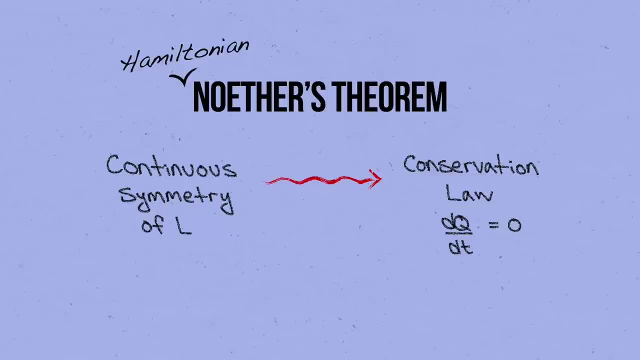 we need to look at things from the perspective of Hamiltonian mechanics, where the relationship between symmetries and conservation laws takes on its most beautiful form. In particular, you might have wondered if the connection goes both ways. Does a conservation law, conversely, imply a? 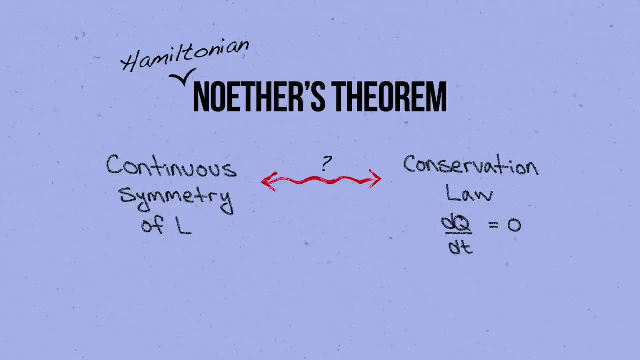 corresponding symmetry In the Hamiltonian formulation of Noether's theorem, we'll see that the answer is quite generally yes. Continuous symmetries and conservation laws go hand in hand. It's hard to overstate the importance of this relationship, both in classical mechanics. 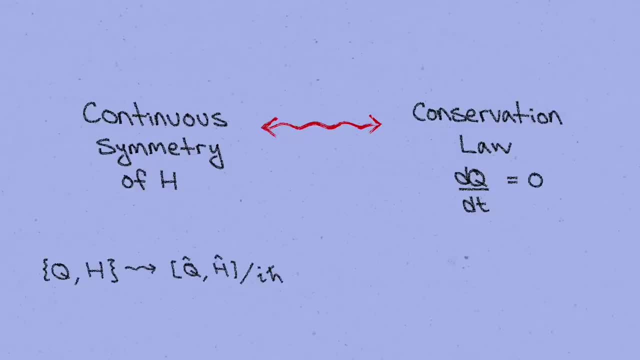 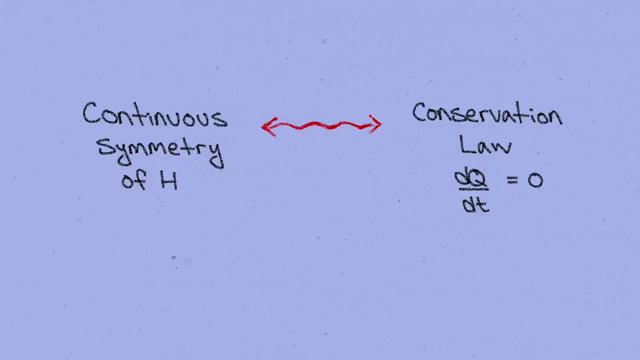 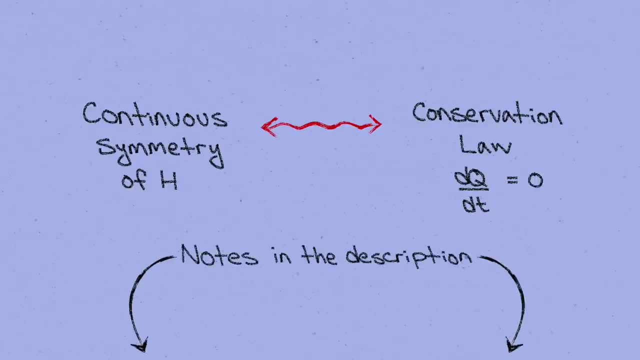 description to help you work through all the details after you've watched. Let's think about a particle of mass m moving in one dimension with coordinate x. According to Newton's second law, the rate of change of the particle's momentum is equal to the total force that's acting on it and the force 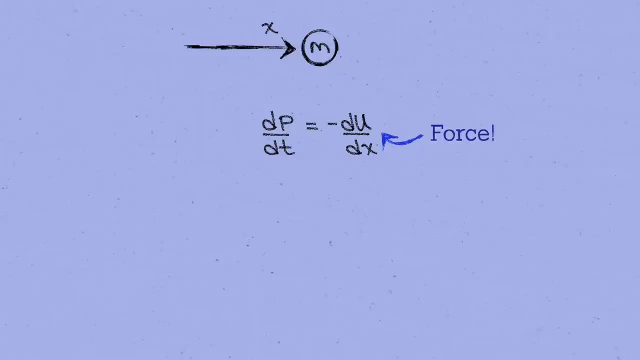 can alternatively be expressed as: minus the slope of the potential energy function. The momentum here is of course defined as the mass times, the velocity of the particle, or flipping that around, dx by dt equals p over m. We can describe what the particle is doing at any instant in time by giving its position and. 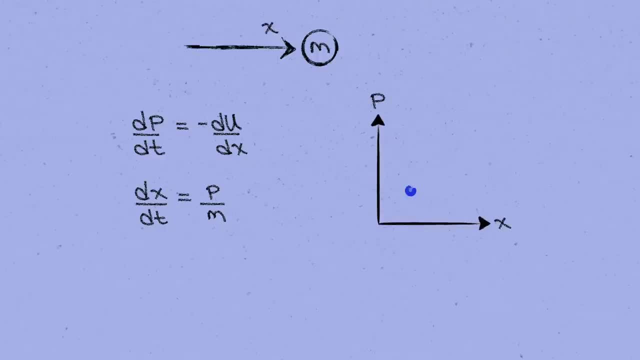 momentum, Then the state of the particle is specified by a point in the xp plane which is called the phase space of the system. As time goes on, the particle moves around and accelerates, and so the corresponding point in phase space also changes The curve that's traced. 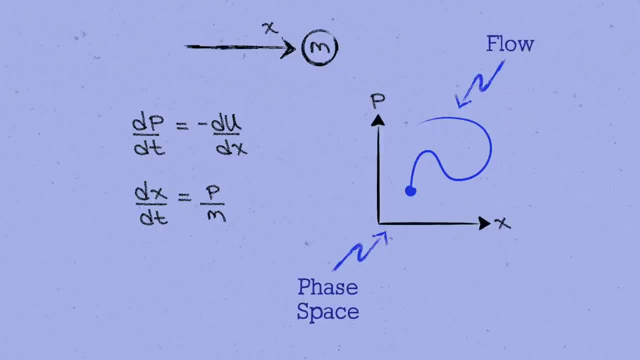 out as this point moves around with time is called a flow on phase space. Think of it literally like the flow of a bit of water along the current in a river. We start at some initial point: x0,, p0, and then these equations for dx by dt and dp by dt. 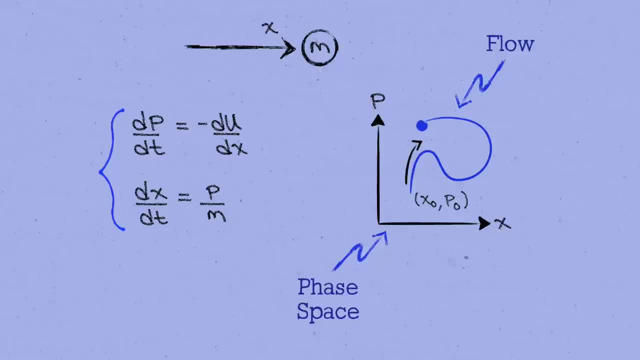 tell us how the current carries this point along through the phase space, giving us a curve with coordinates x of t and p of t that we call the flow. I showed you in another recent video that we can rewrite these equations in a very compact way using Poisson brackets. 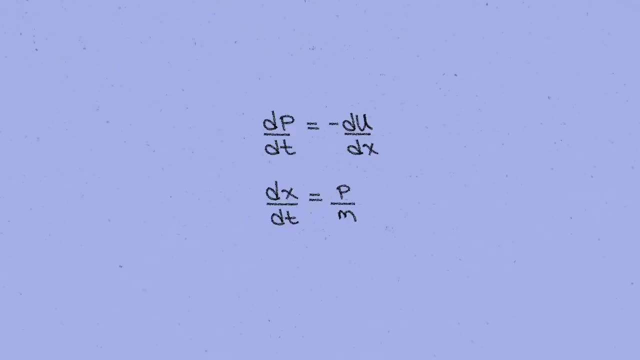 Which, in turn, are essential for understanding the parallels of these classical ideas in quantum mechanics. I'll link that video up in the corner if you haven't seen it yet. We showed that the rate of change of x is just given by its Poisson bracket with the hamiltonian. 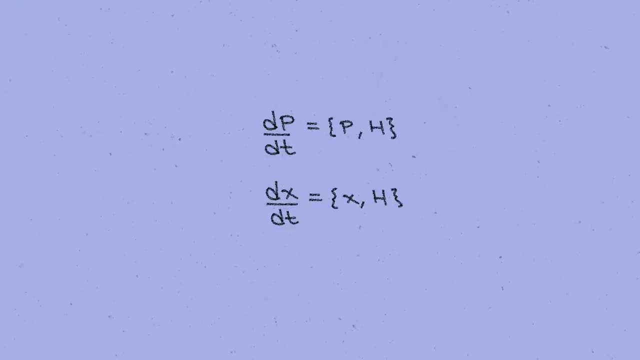 h, And likewise the rate of change of p is given by its bracket with h. H. here is the Hamiltonian function, which in simple circumstances is just the total energy, and we defined the Poisson bracket as a kind of anti-symmetric combination of derivatives with respect to x and p. 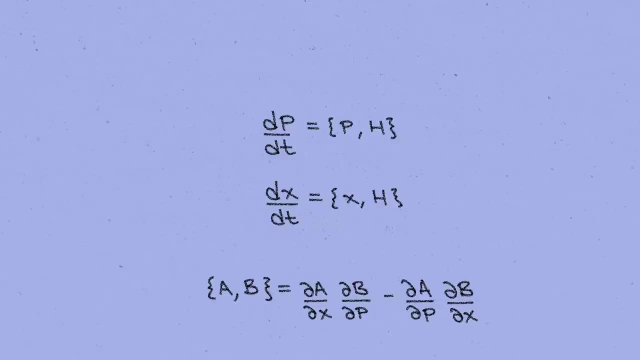 It's the derivative of the first thing with respect to x times the derivative of the second thing with respect to p, minus the reverse derivative, with respect to p, of the first thing times the derivative of the second thing with respect to x. 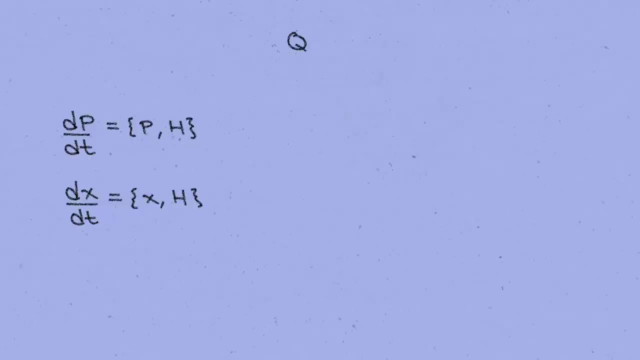 In fact we prove something more general, that for any function q on phase space, its rate of change with time is given by the Poisson bracket with the Hamiltonian. You can choose any quantity q that you like here. the position x, momentum, p, the Hamiltonian. 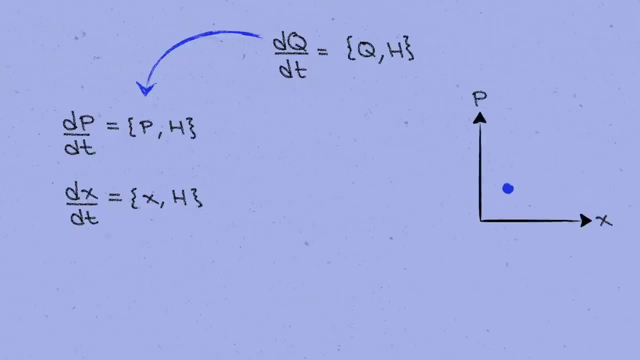 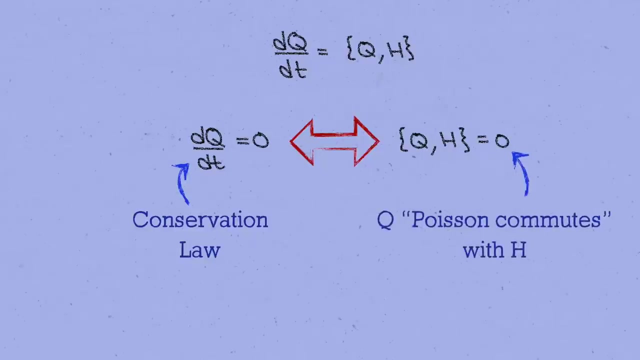 h or whatever else, and this formula tells you how it will change as you follow along the flow. This gives us a simple condition for determining: if a quantity q is conserved, its Poisson bracket with the Hamiltonian must vanish. We say that conserved quantities Poisson commute with the Hamiltonian. 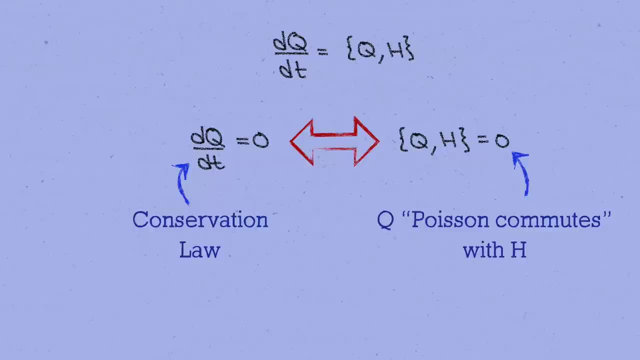 So that tells us how to understand conservation laws and Hamiltonian mechanics. Now the question is: how does all this relate back to symmetries? That's what I want to explain in the second half of the video. To understand it, we have to break down what the heck it really means physically for a function on phase. 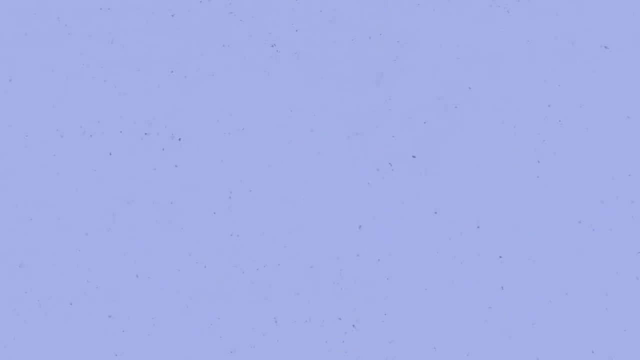 space to Poisson commute with the Hamiltonian. The fact is, the mathematical framework of Hamiltonian mechanics in terms of flows on phase space is much more general. The flow equations determine how the phase space point moves around with time, But mathematically there's nothing particularly special about the Hamiltonian. 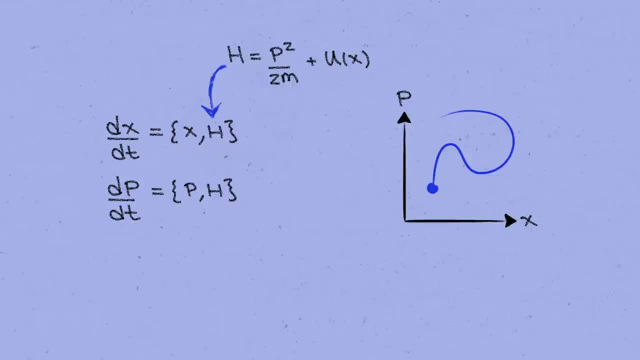 It's just some function h on this space. Physically, of course, it's very significant, But the point is that mathematically, the Hamiltonian is a function of the Hamiltonian and the Hamiltonian is a function of the Hamiltonian. 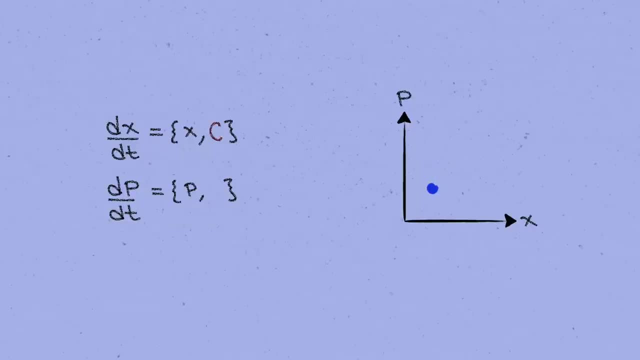 We can just as well define a flow associated to any function. call it g, say on phase space. When we solve these equations, we get some other curve in the xp plane, In fact, since this new flow won't have anything to do with how the particle is changing with. 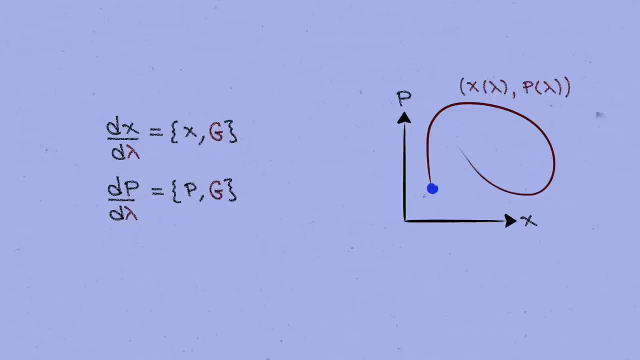 time. let me rewrite the parameter along the curve as lambda instead of t, where lambda is some arbitrary parameter. We call the function g the generator of the flow that's obtained by solving these equations. The curve that you get will depend on what you choose for g. 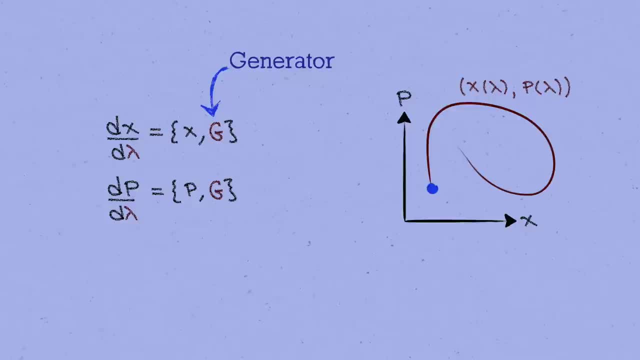 So far we've chosen g equals h to be the Hamiltonian. Then we just get back our old f equals ma equations and the resulting flow describes how our initial point moves around with time. We therefore say that the Hamiltonian is the generator of time translations. 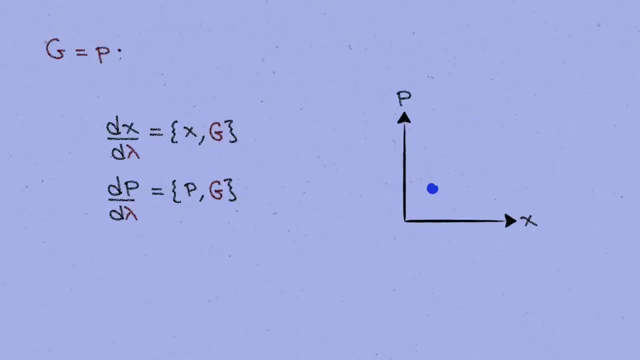 But let's try a different choice. Say we set g equals p to be the momentum, Then what flow is defined by the corresponding equations And, more importantly, what is the physical significance of it? If we plug these into the definition of the Poisson bracket, we get x bracket, p equals. 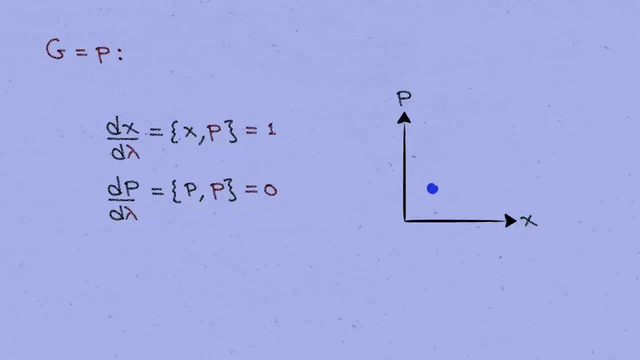 1, and p bracket p equals 0. So these are actually pretty simple as far as differential equations go. Again, picture this like the flow of a bit of water along the current in a river. We start at some initial point- x0,, p0,- and then this pair of equations tells us how the 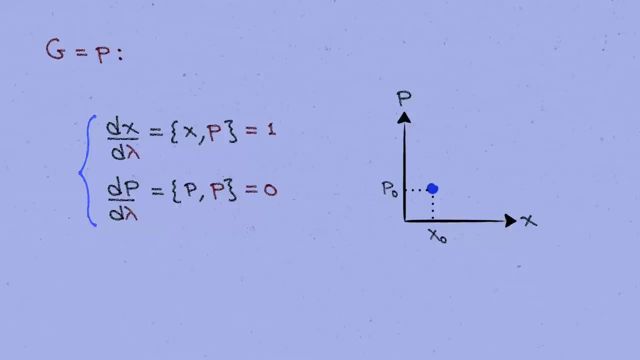 current carries it around as we evolve the parameter lambda. The second one just says that p is constant along the flow. p of lambda equals p0. So whatever momentum p0 that you started with, it never changes along the flow and you're. 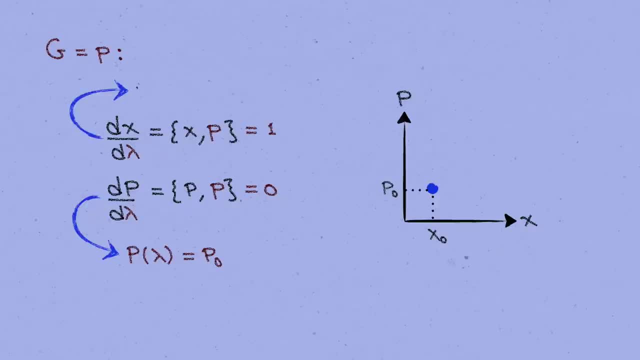 stuck on that horizontal line in phase space. The first equation meanwhile says that x of lambda is a straight line with slope 1, x of lambda equals x0 plus lambda. So we start at position x0 and then get shifted over by lambda. 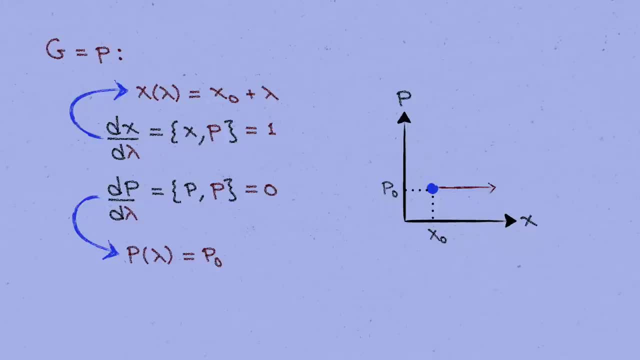 So this flow says: to translate the position, coordinate over by lambda and leave the momentum coordinate alone. Then the flow on phase space generated by p isn't such an abstract mathematical curiosity, after all. It just describes a spatial translation. It picks up the particle and shifts it over a bit. 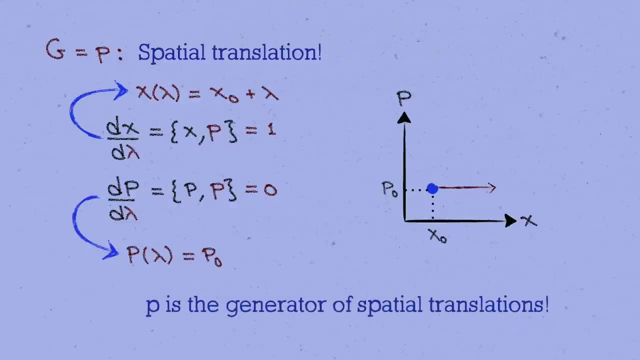 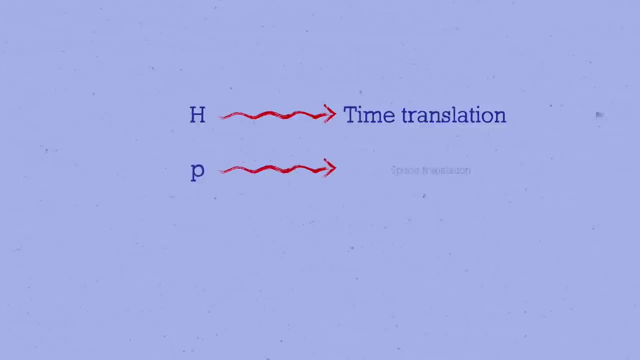 We say that momentum is the generator of spatial translations, Then in the same way that the Hamiltonian h generates time translations, we've learned that the momentum p generates spatial translations. And likewise, when we step up to more than one dimension, the angular momentum l will. 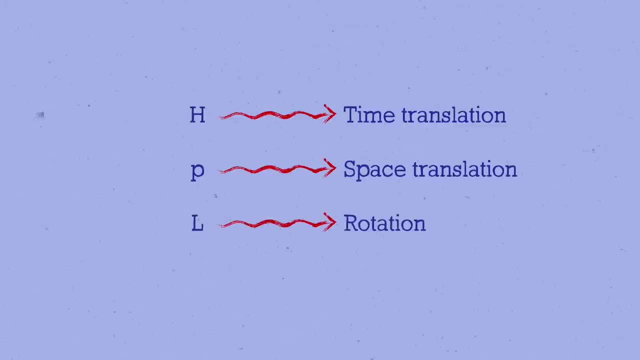 generate rotations. But we saw in the video about Noether's theorem that when these transformations are symmetries, they lead to corresponding conservation laws. Time translation invariance leads to spatial transformations. It leads to energy conservation. Space translation invariance to momentum conservation. 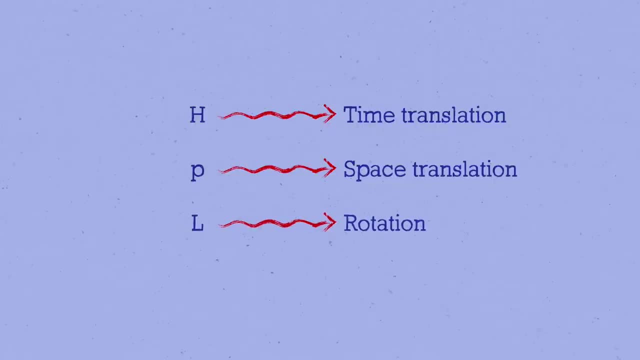 And rotation invariance to angular momentum conservation. And now we're ready to bring it home and understand these relationships and Hamiltonian mechanics And in fact to discover that the connection goes both ways: The symmetry implies a conservation law and the conservation law implies a symmetry. 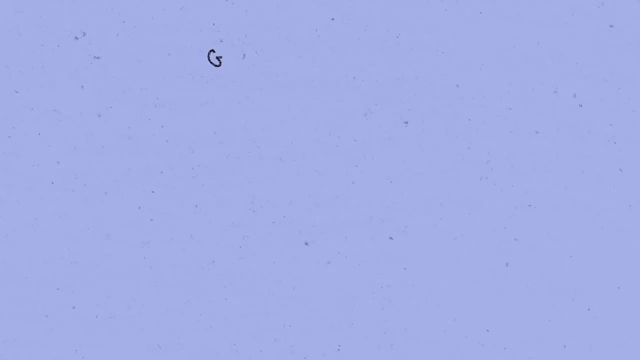 We've seen that any function g defines a flow on phase space, And likewise that the rate of change of any other function q along that flow is given by its Poisson bracket with the generator g. Now let's go back to g equals h, so that this equation says how q changes with time. 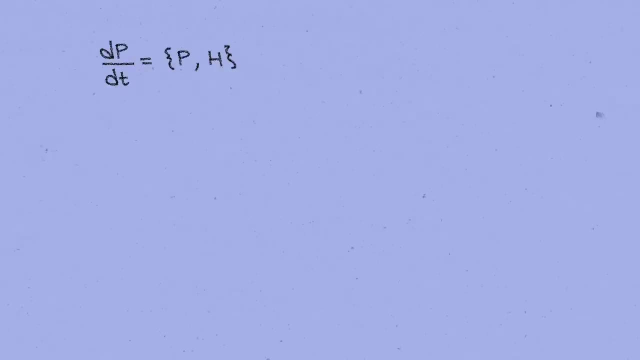 And for concreteness sake let's pick our quantity q to equal the momentum p. Suppose we have a system where the momentum is conserved, which for a single particle would require that it's free. But all of this of course generalizes to systems with multiple particles and multiple dimensions. 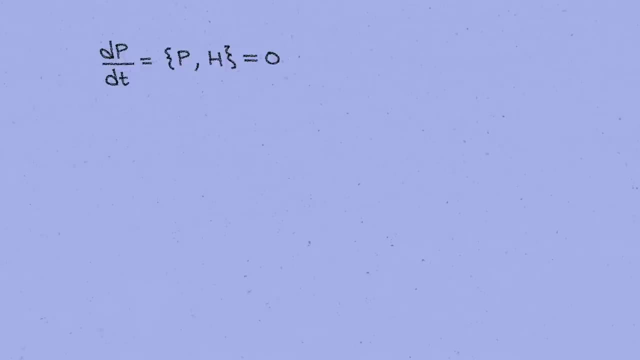 Then dp by dt equals zero. In our fancy new language we'd say that p is invariant under the flow generated by a- h, But we've learned that we can just as well consider the flow generated by p. it's simply a spatial translation. 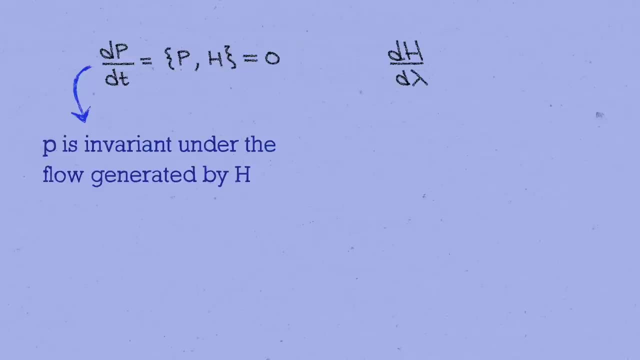 And the rate of change of h along the flow generated by p is given by dh. by d, lambda equals h bracket p. Now, Poisson brackets are anti-symmetric, meaning that a bracket b equals minus b bracket a, as you can check from the definition. 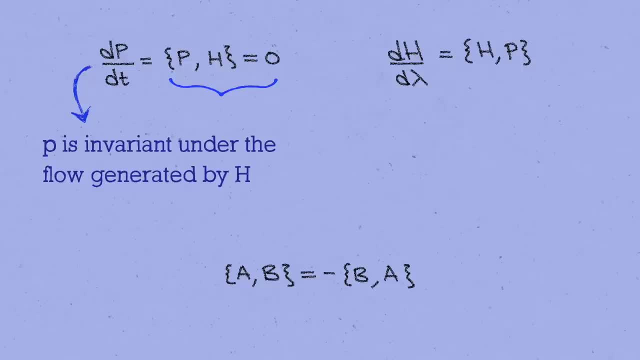 And so if p bracket h equals zero because p is a conserved quantity, then likewise h bracket p will vanish, Which in turn means that p is a conserved quantity, Which in turn means that h is invariant under the flow generated by p, which again is just. 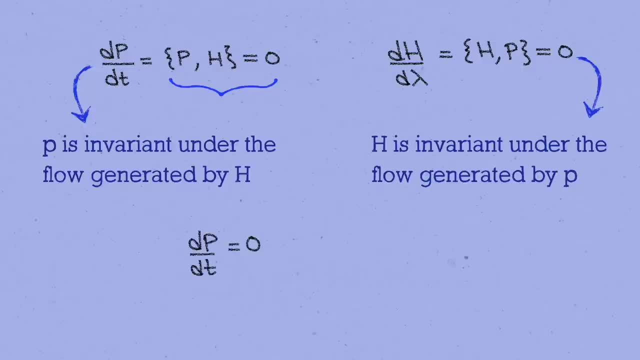 a spatial translation. Thus, the momentum will be conserved if, and only if, the Hamiltonian is invariant under spatial translations, In other words, if translations in space are a symmetry. This is the Hamiltonian version of Noether's theorem: A quantity is conserved if, and only if, the transformation that it generates is a symmetry. 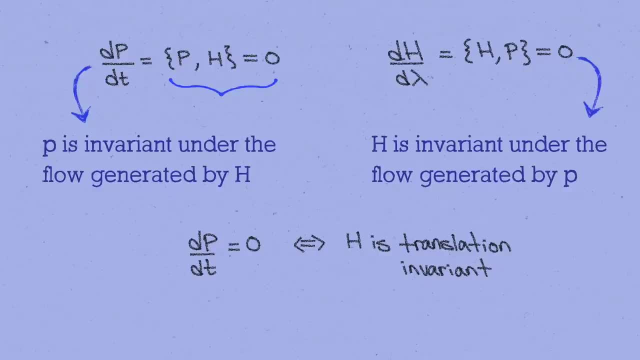 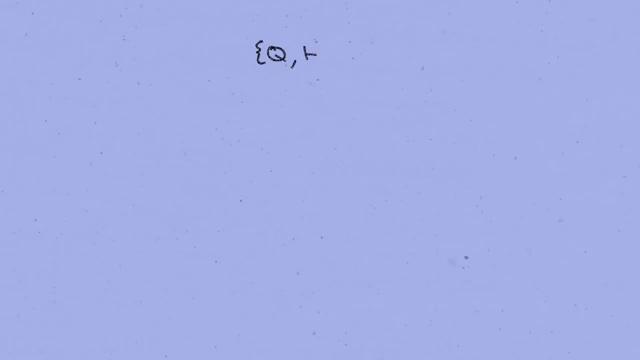 of the Hamiltonian. That was the punchline, And I think it's a challenging one, So let me say it again for the general case, A quantity q will be conserved in time if its Poisson bracket with the Hamiltonian vanishes. 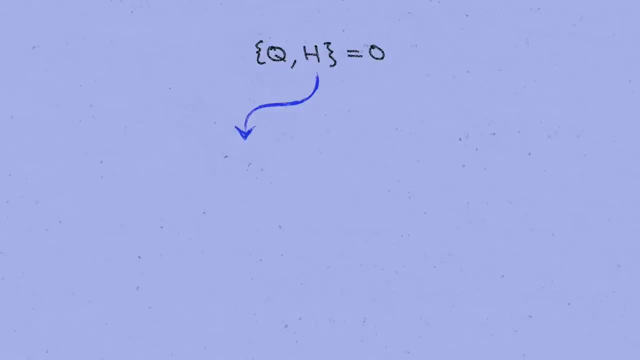 But there are two ways of interpreting this bracket. First, like we have here, as the rate of change of q along the flow generated by h, But second, up to a minus sign, q. bracket h is likewise the rate of change of h along. 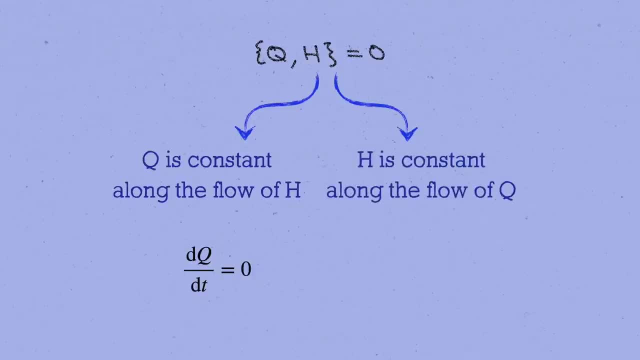 the flow generated by q. So q will be conserved in time if, and only if, the Hamiltonian is invariant under the flow generated by q, That is, if the transformation generated by q is a symmetry. In this way, the correspondence between symmetries and conservation laws follows from these two. 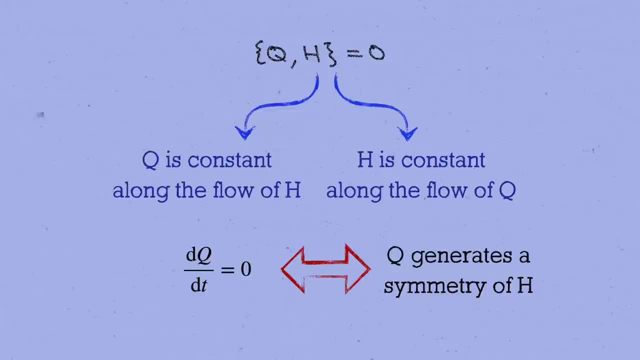 reciprocal interpretations of our simple equation for the rate of change given by the Poisson bracket. The two interpretations are physically very different, though The flow generated by h is about how the system changes with time. The flow generated by q is the symmetry transformation, like picking up the system and sliding it. 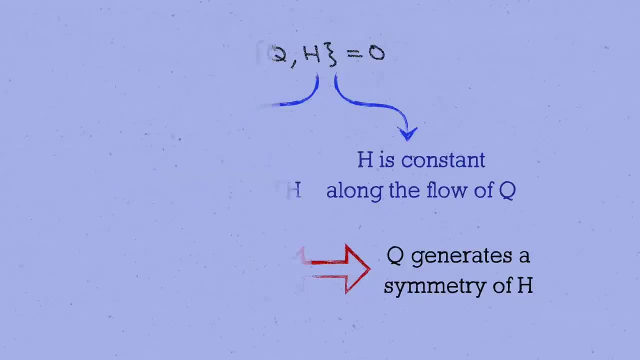 over or rotating it around. I'll wrap up by mentioning a couple of tidbits that we might get to explore more in future videos, if you're interested. The Poisson bracket is a very special operation and it defines a mathematical structure called a Lie algebra on the set of functions on phase space. 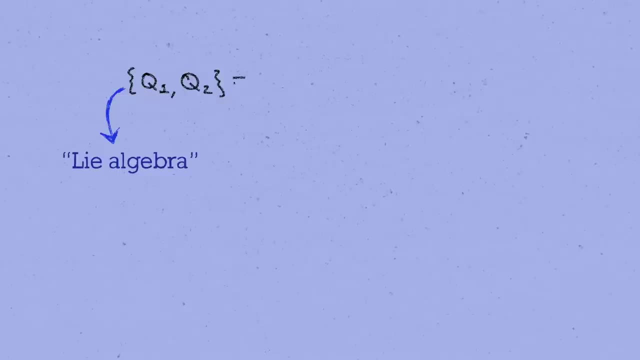 You can show that the Poisson bracket of two conserved quantities is itself conserved and therefore the set of conserved quantities form what we call the symmetry algebra of the theory. The classic example comes from the components of the angular momentum vector. If you plug them into the Poisson bracket you'll find that their symmetry algebra.